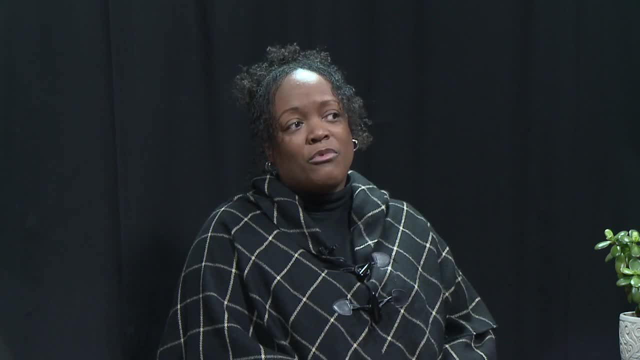 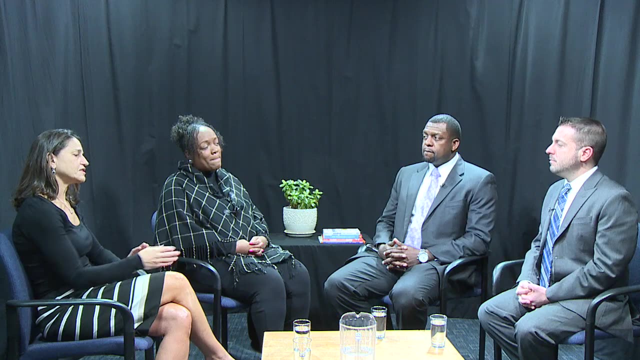 things that are happening in our building. Those were major shifts for us in Greece and I think that everyone is stepping up for the challenge. And, as an instructional coach, have you seen that translate to changes in the student behavior? Yeah, absolutely. 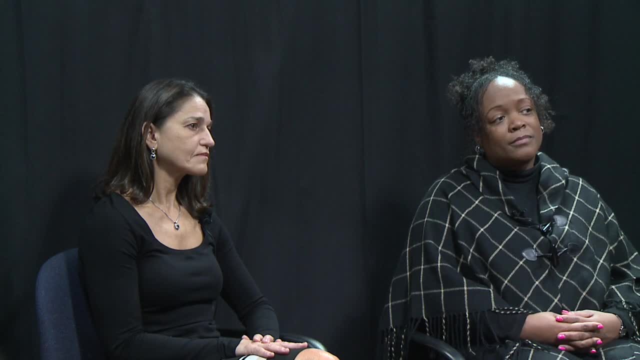 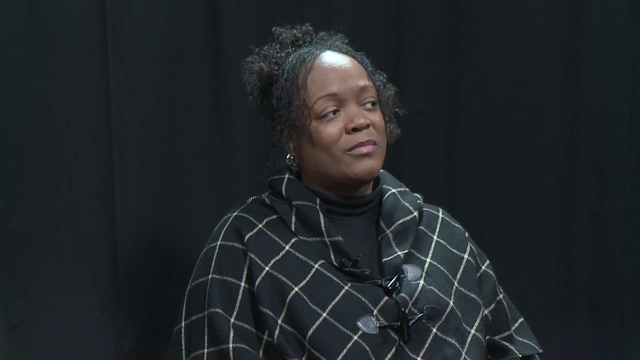 As a coach or teacher leader. you're going into a classroom and you end up working with kids because that's your natural instinct as a teacher. So what's nice about that is you see instruction in one classroom that's strong, And then you go and work with a teacher down the hall or in another building, or you. 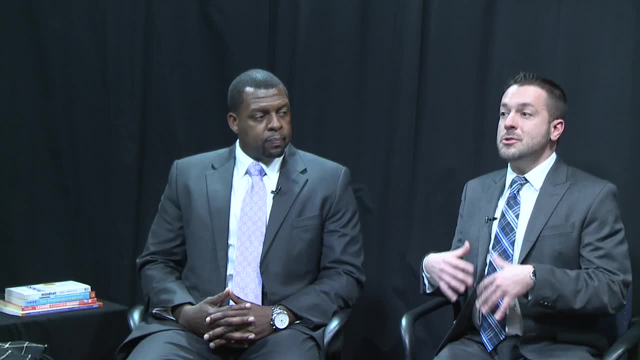 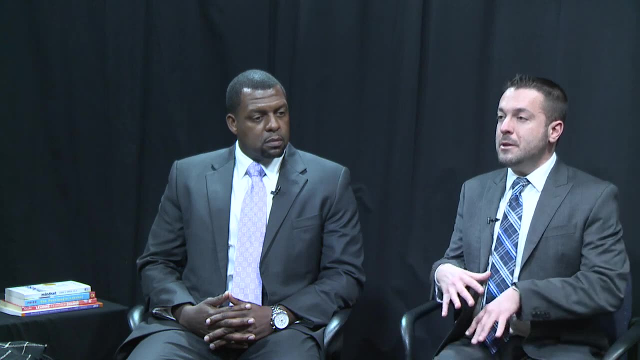 go talk to the administrators, the superintendents, and you say: this is really great, Or here's a pocket that could use a little more support. So there's consistency amongst the buildings and there's a better, I would say, communication. 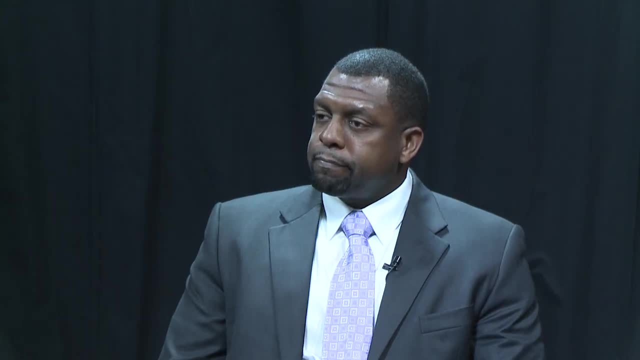 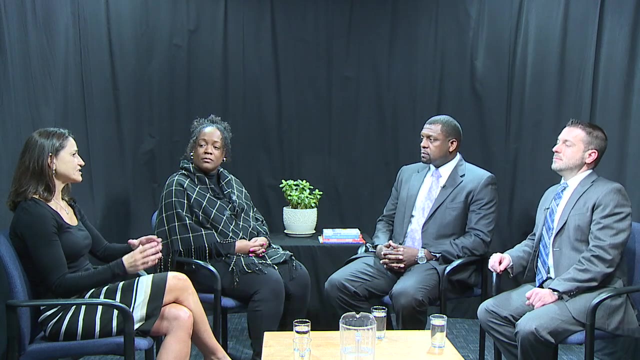 chain for instruction across the district. So I think that consistency is the theme really And I know as an instructional coach in Huntington I see that as well. You know, when I go from class to class the students feel that consistency. 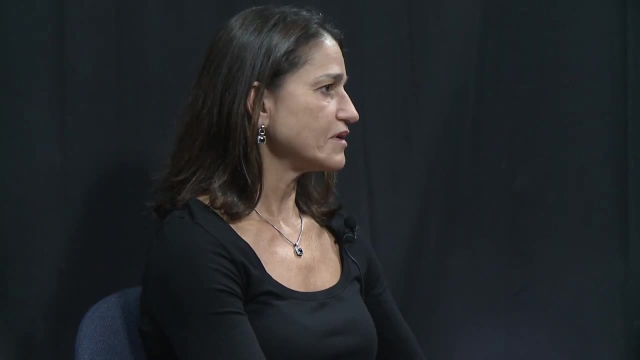 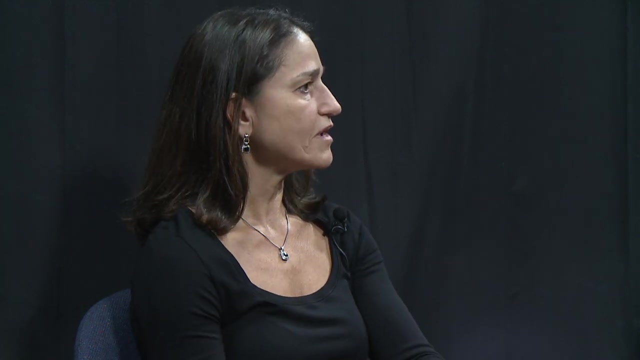 And they realize that not only the things that they are doing in perhaps, their English language arts class will happen there, but it also happens in their science classroom and in their math, And the language is the same and the level of instruction is the same. 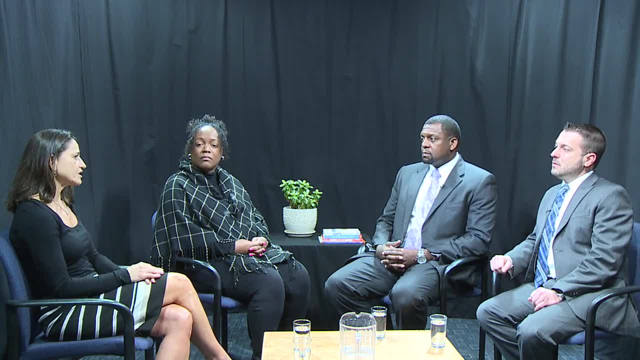 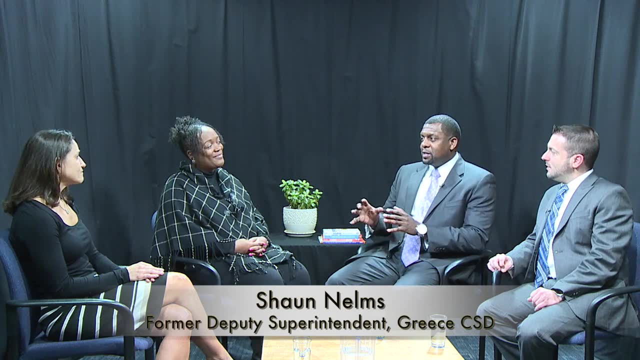 And so it's really that consistency that's really raising the bar here for the students in the schools. It's always great when you walk into a classroom and you hear a student say things like this reminds me of what we did in this classroom, or last year we did this. 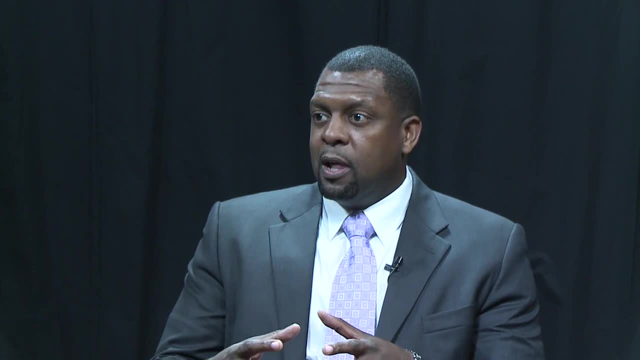 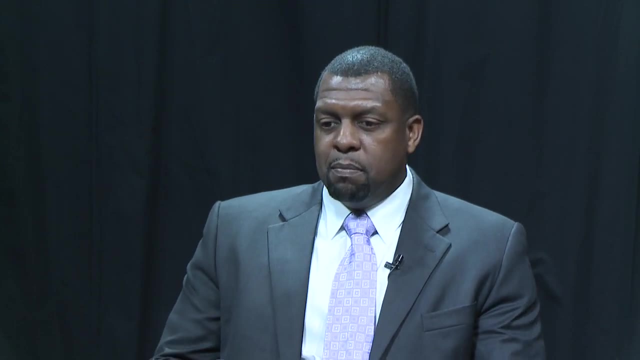 And students are making these natural connections Because the teachers are planning purposefully. They're no longer disjointed. When I say team, it's a true team. You walk into our PLCs and to have an administrator not be the person doing the talking but listening. 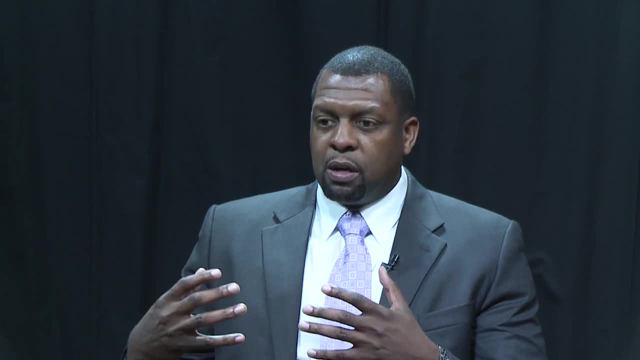 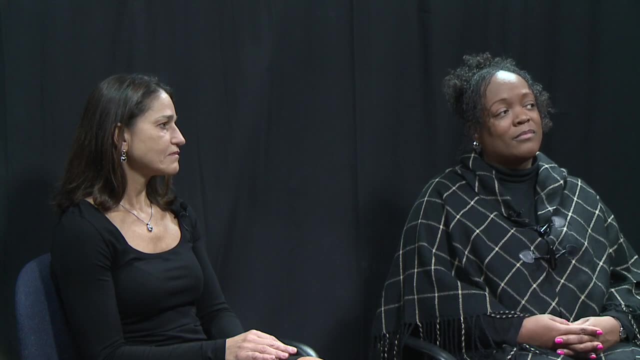 and just facilitating the conversation, having these teachers share things that are working, sharing concerns and then identifying solutions. In the past, it was a matter of coming to PLCs and talking about problems and leaving them at the table. The administrator walked away, did some guesswork, came back and they started all over again. 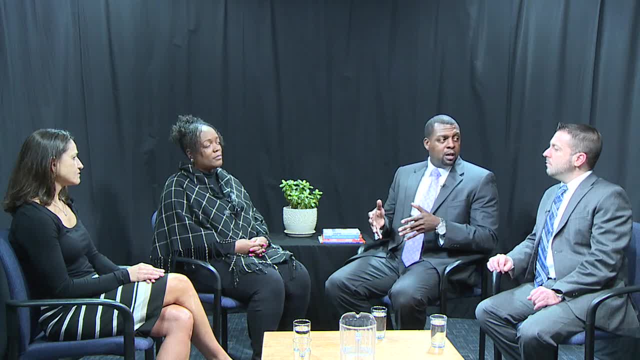 You're seeing issues emerge and be resolved right there, on the spot. As you said, it's on demand, It's real, And then it allows you to go back and check that And then those solutions are shared across the system to prevent other teachers from. making those same pitfalls. It's a really encouraging environment right now. 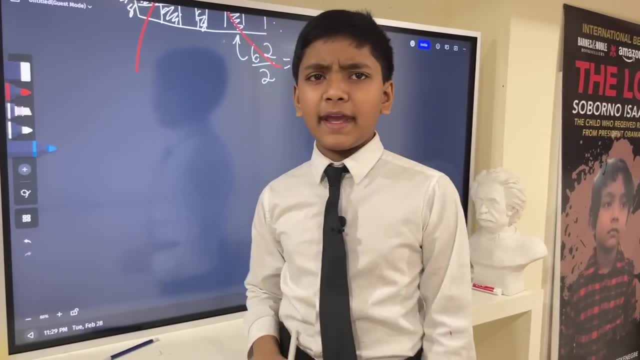 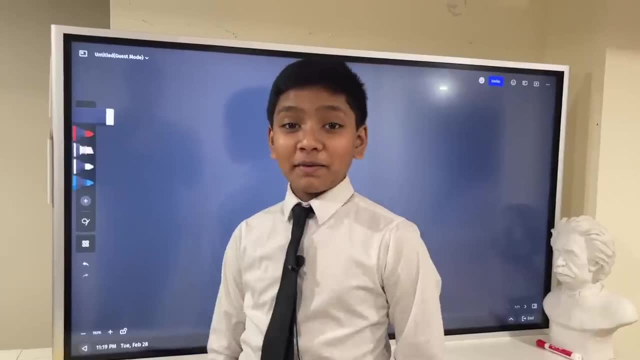 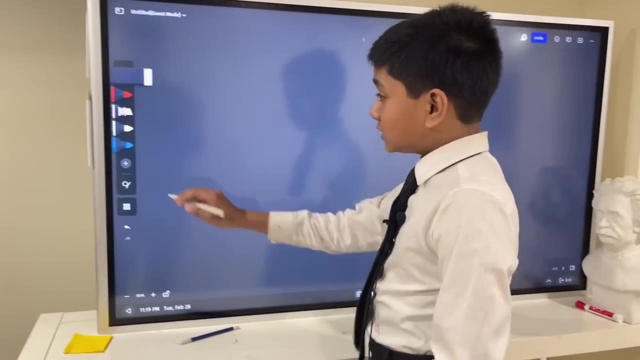 Let's say: Baby, you want to do it tomorrow? Mm-mm. Okay, Hello everybody, My name is Abonai Isaac-Bearer from BearScienceLab, And today I just wanted to talk to you about a really cool new concept that I just discovered called the pigeonhole principle. 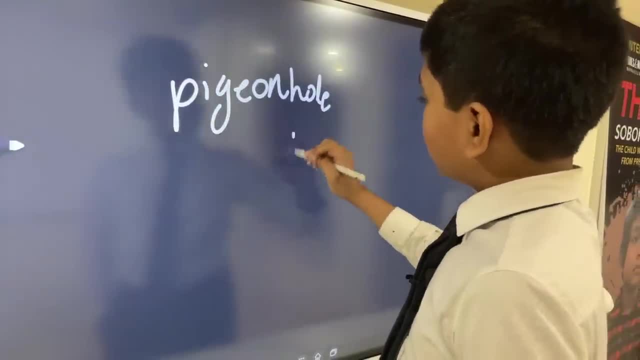 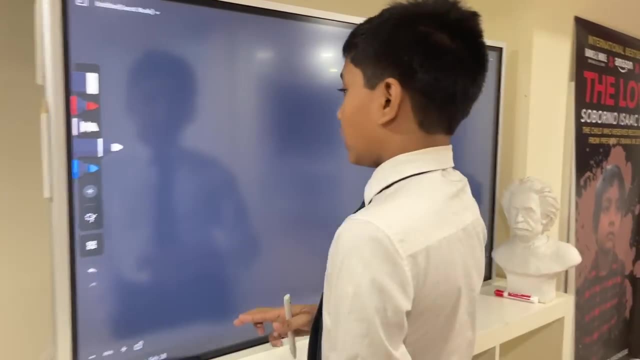 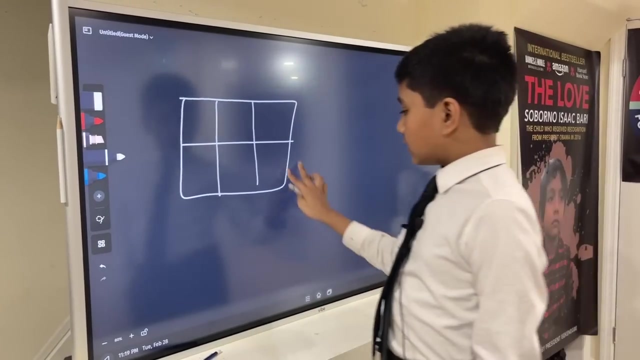 Yes, the pigeonhole principle. So basically this is what it says. Let's say you have- I don't know- six holes, And let's say you have, Let me draw a pigeon real quick. So here's our pigeon. 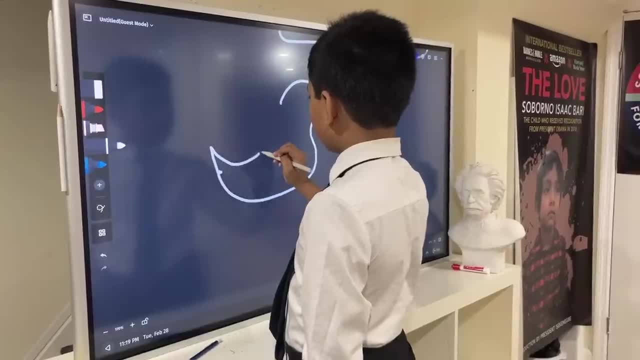 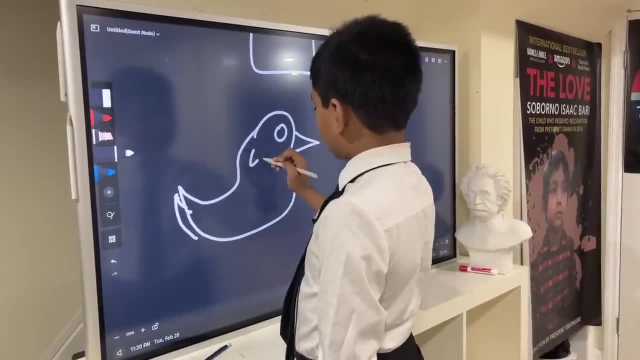 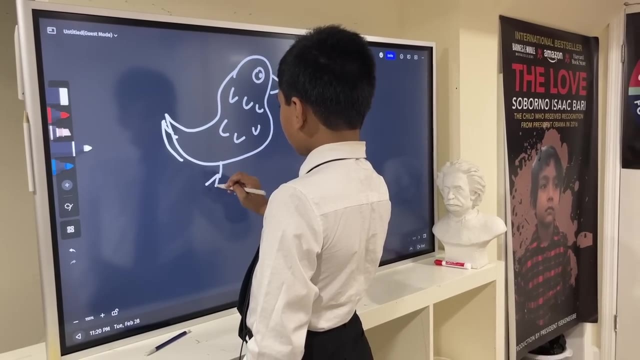 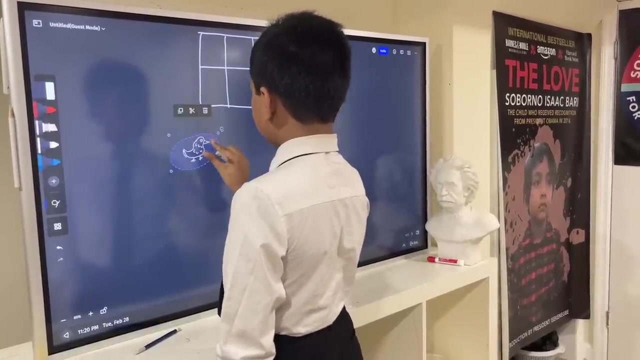 I'm going to make it a little chubby. I know it looks like a duck right now, But trust me, it's a pigeon. So this is just like some stuff. So here is our pigeon, right, And so what I'm going to do is let's say we don't have just one of these. 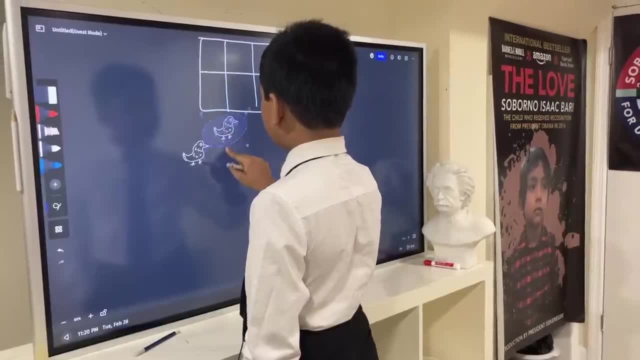 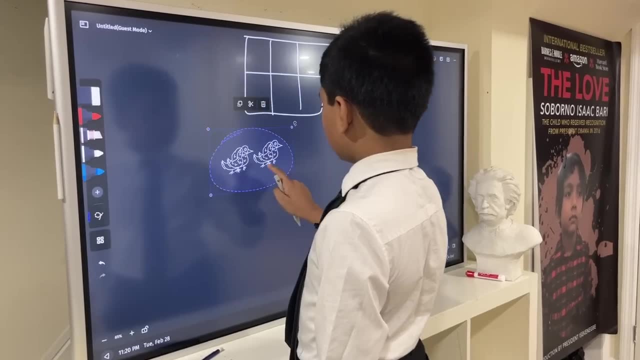 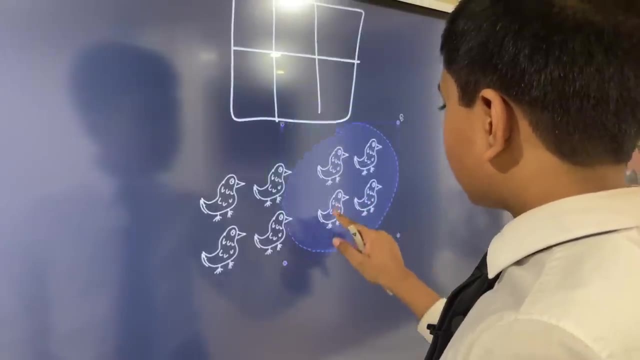 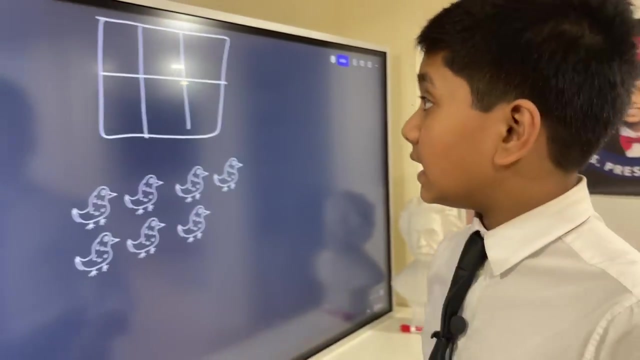 But let's say we have seven, So two, Let's copy that Four, Let's copy that Eight, And now So we just erase. So this is what the principle says. We have seven pigeons and six boxes. 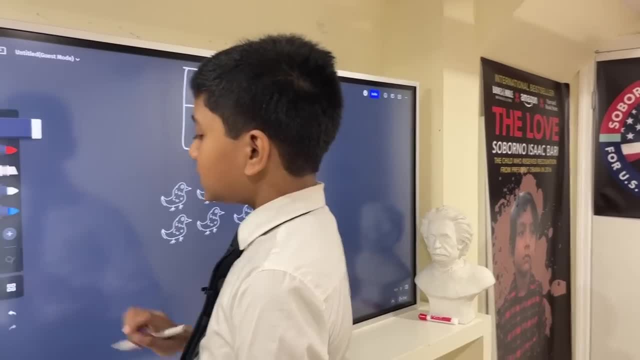 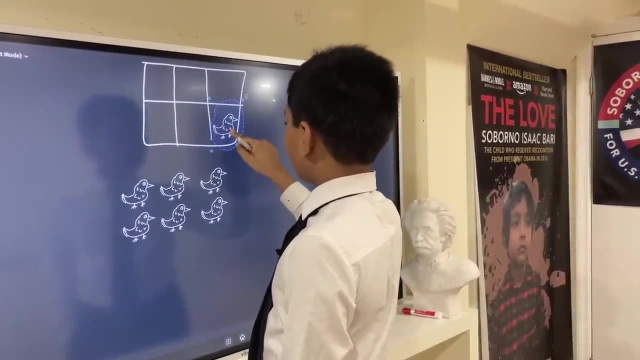 So this might seem quite obvious, But that means that at least one of these boxes has to have more than one pigeon in it. So if I try arranging them, Let's just shrink them down a little bit more so that they fit in the box. 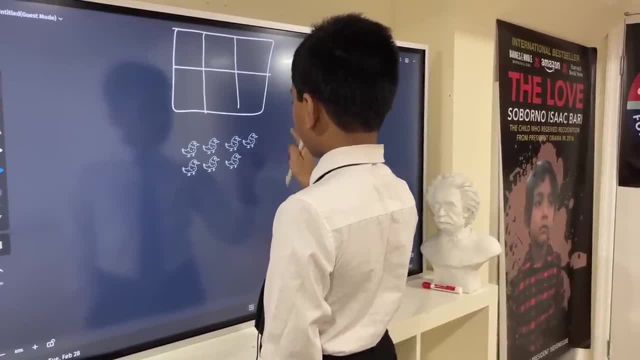 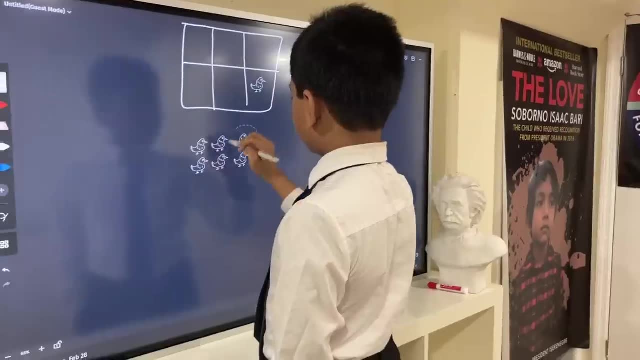 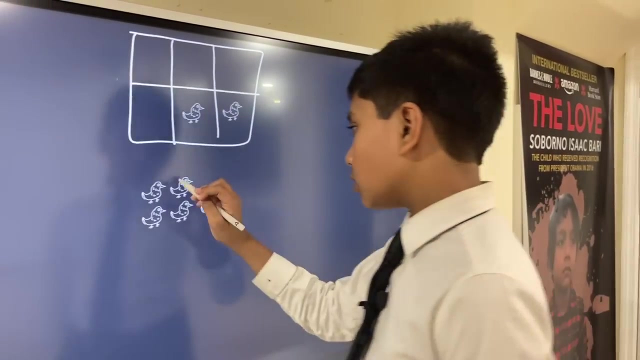 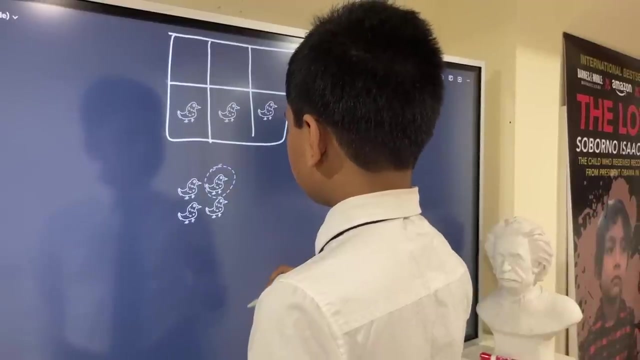 Sliding a little bit. So let's, Let's try arranging them. Hmm, So if we put one pigeon in here, let's say: Why is it so laggy? One pigeon in here, One pigeon in here, One pigeon in here.